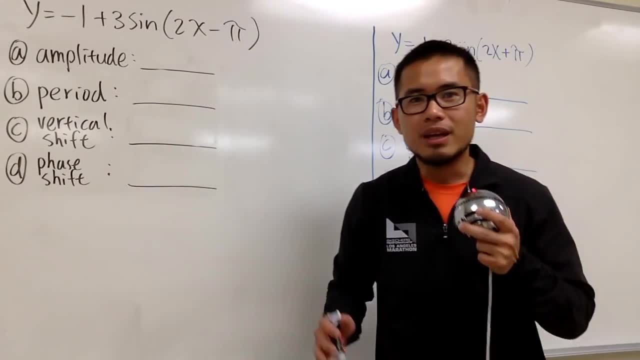 In this video I will show you guys how to find the amplitude, the period, the vertical shift and also the phase shift for a sine function And, more importantly, I will compare and contrast these two equations here and I'll point out all the details that you have to remember. 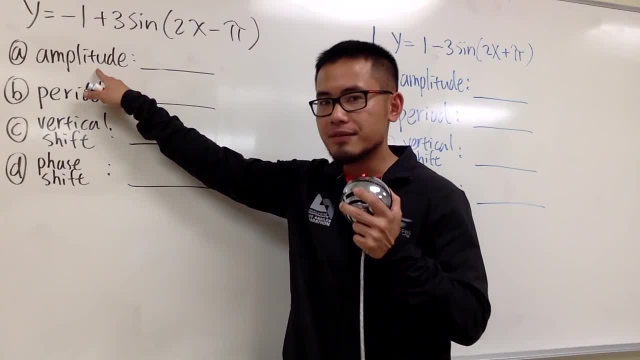 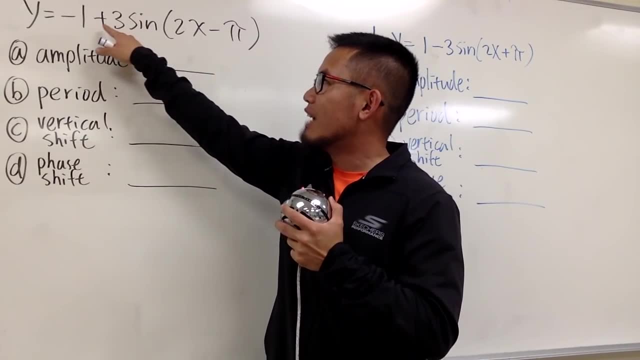 Let's focus on this one right here. So let's go ahead and identify the amplitude. This is just going to be the absolute value of the coefficient of the sine. So, as we can see, we have a positive street right here. Remember, for the amplitude, you always take the absolute value. 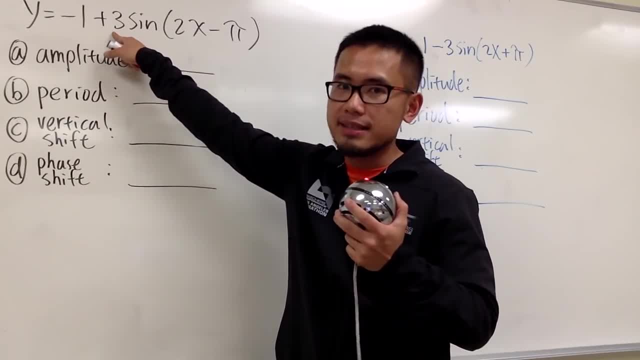 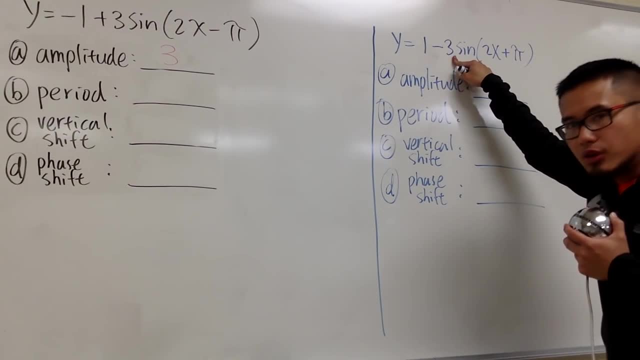 So the absolute value of a positive street will still end up with a positive street. So this is it all right? Well, what if we had a negative street right here For the amplitude? remember we have to take the absolute value for that. 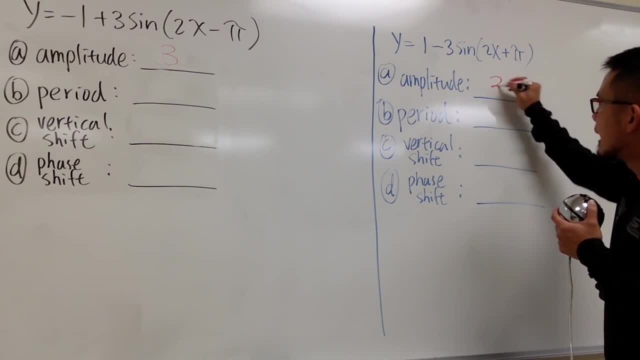 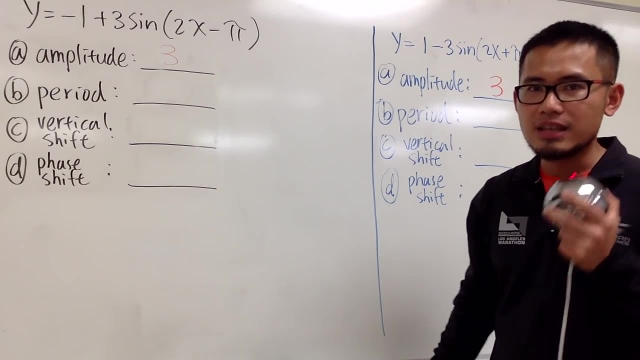 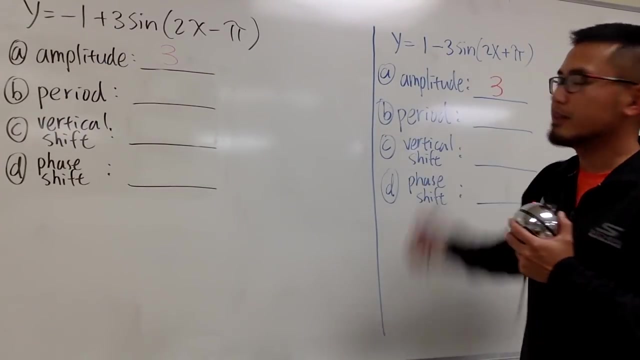 In this case, here the amplitude is still going to be positive street, all right. So remember the amplitude, the answer to the amplitude, it's always going to be a positive answer. okay, Positive answer. So we have to take the absolute value of the positive street right here, regardless to the sine, either plus or minus, that they have in between. all right, 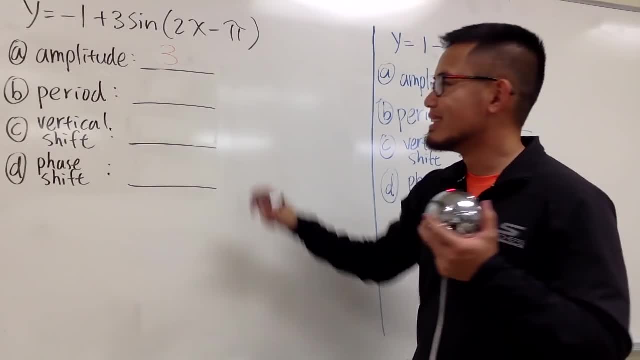 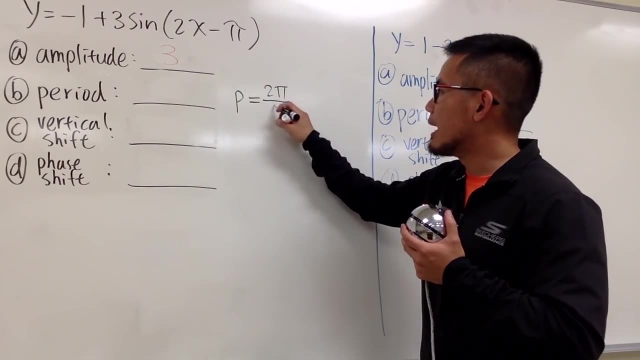 Next we are going to find the period and we have to know the formula. all right, So let me just put on p for the period. This is going to be 2 pi- it's always 2 pi on the top- and divide it by the b value. 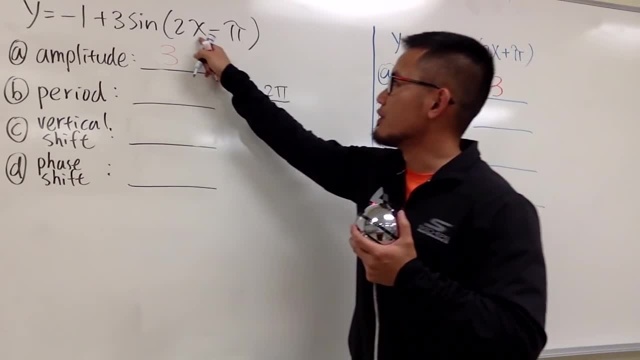 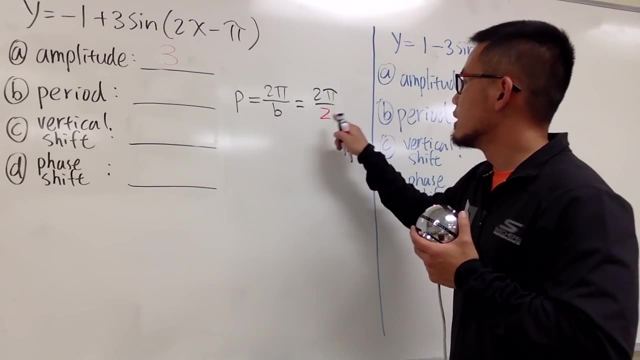 So what is b? b is just the number in front of the x. In our case it is positive 2.. So this is just going to be 2 pi over 2.. This 2 is positive, So we have 2 right here, okay. 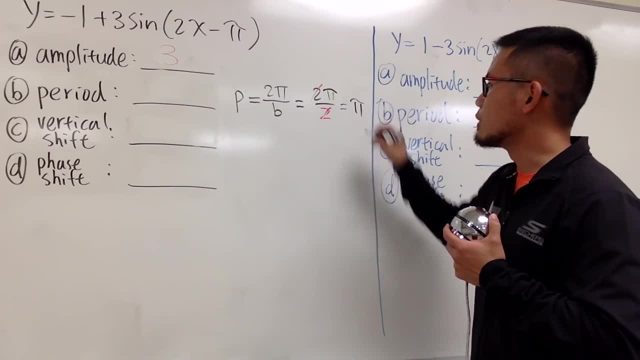 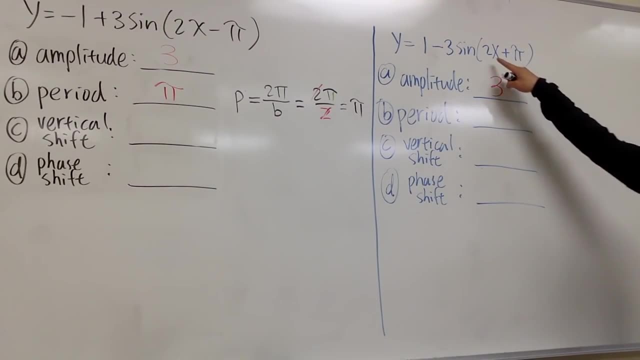 And of course you can see that 2 and 2 cancel, so altogether we just end up with pi. So for this one the period is just pi, And in this case here because the b value is the same, so the period right here is also just going to be 2 pi over 2 right here. so it's still going to be just pi, right? 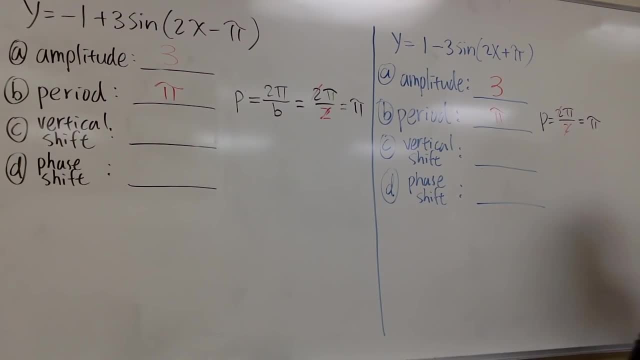 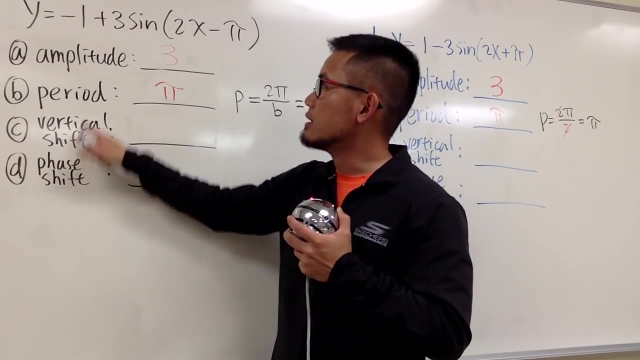 So we have pi right here as well, like that. Okay, next, vertical shift. In our case here, the vertical shift is the number all the way in the front, right in this form. So this right here is all the way in the front. 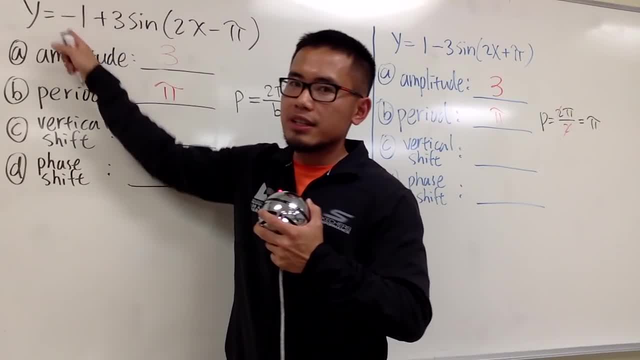 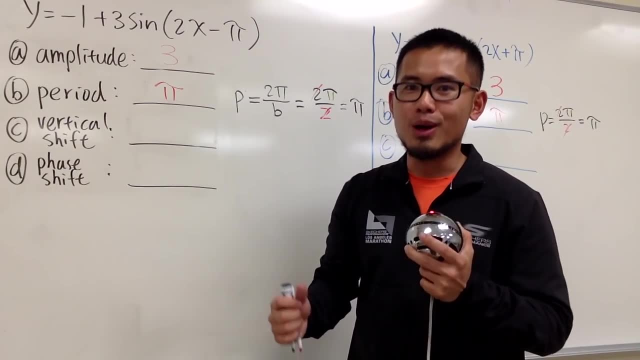 It's not about the sign. all right, Here we have negative 1.. The negative 1 tells us we are going to move the original 1 down below. So this is how you're going to answer it: The vertical shift, you're going to tell me. 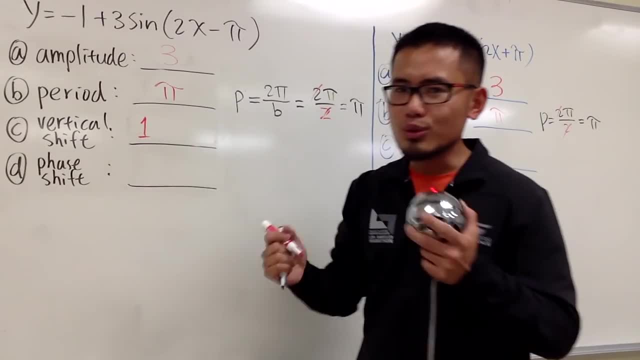 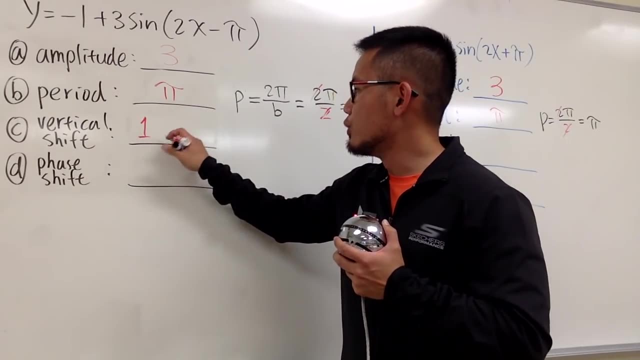 don't just put down negative 1.. We need to know the direction. This negative 1 right here tells us it's 1 unit down below, So 1 unit down. So you can just say 1 unit down or 1 down, something like that. 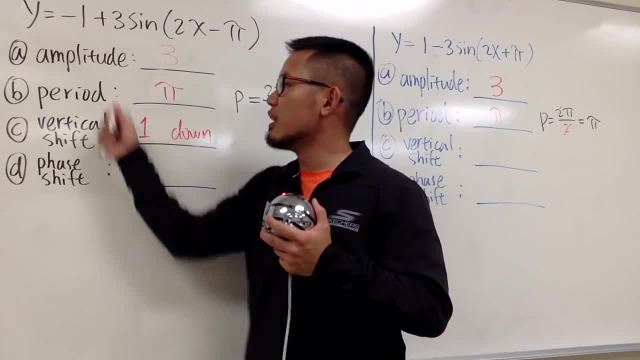 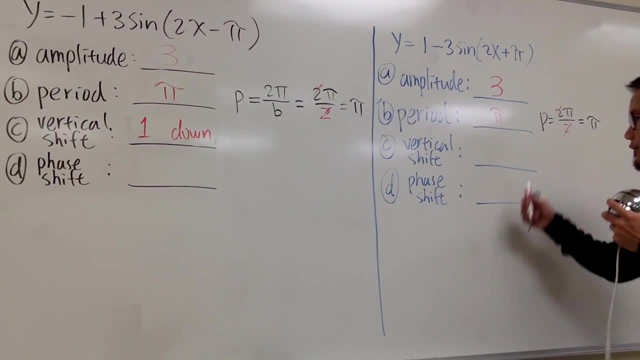 This is good enough? all right, So do not just put down negative 1. Be sure, Just put down the absolute value of whatever that number is and tell me the direction. Okay, for this one vertical shift, if this is the equation. 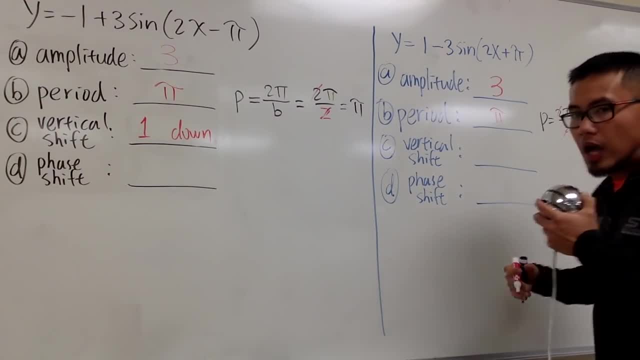 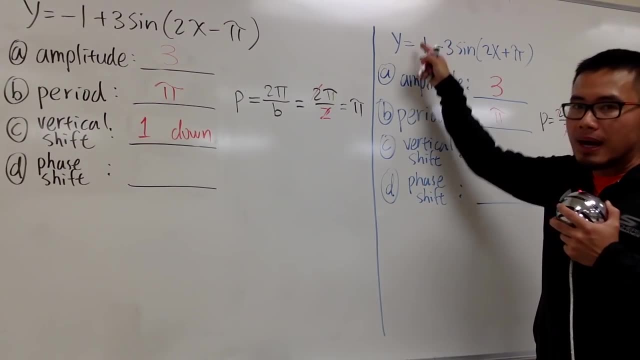 if that was a positive 1,, okay, how many units we are going to move is still going to be 1 unit, right, So we still put down 1.. This time this was a positive 1,, right, So that will tell me it will go up. 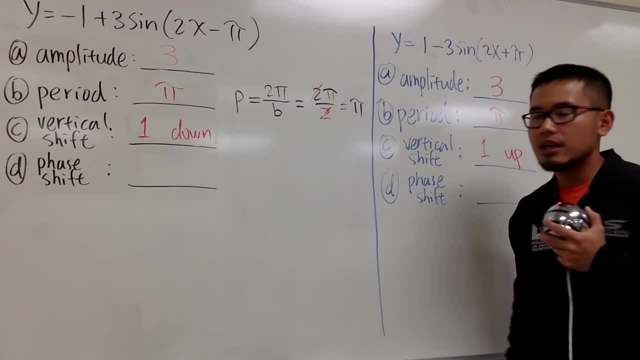 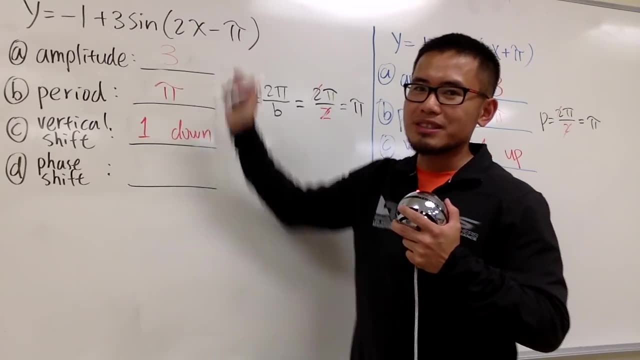 It will go up 1 unit. So that's the difference At the end: phase shift. So the phase shift is something that we have to talk about inside right, And let me just write that down right here. Here's the general form. 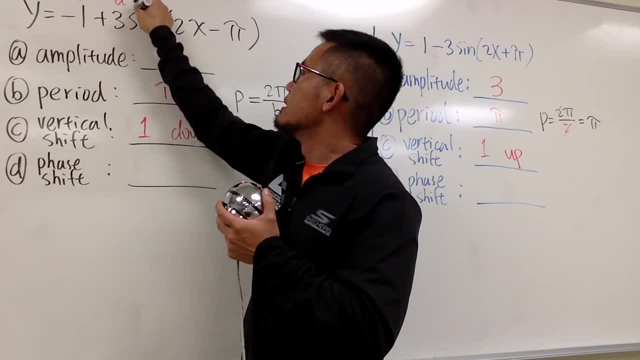 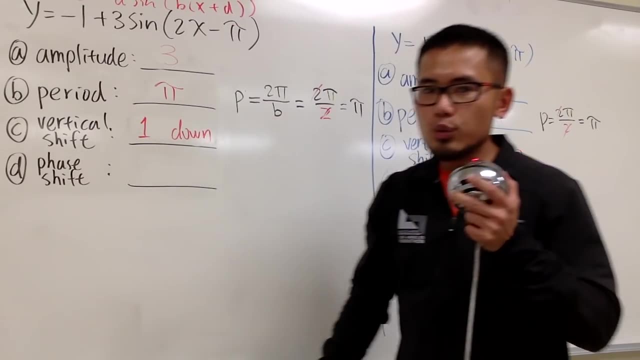 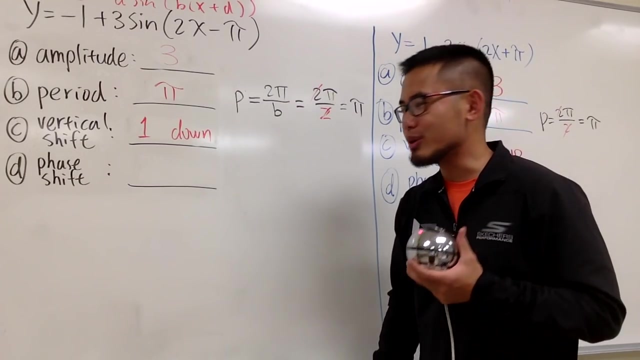 C plus A times, sine of parentheses, B, times the parentheses X plus D. okay, And you see, in order for you to figure out the phase shift, you have to do something with the inside Factor things out. And let me show you how to do it right here. 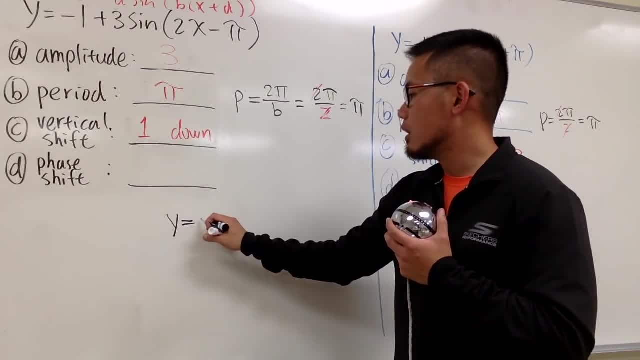 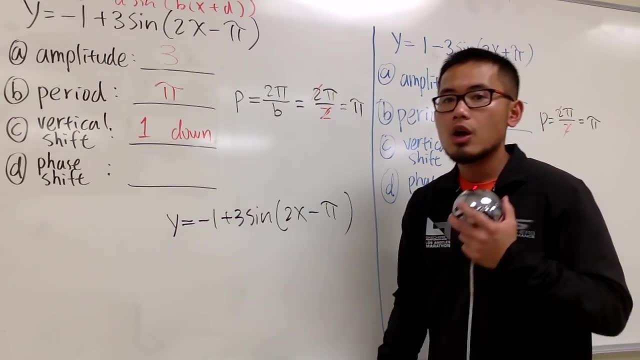 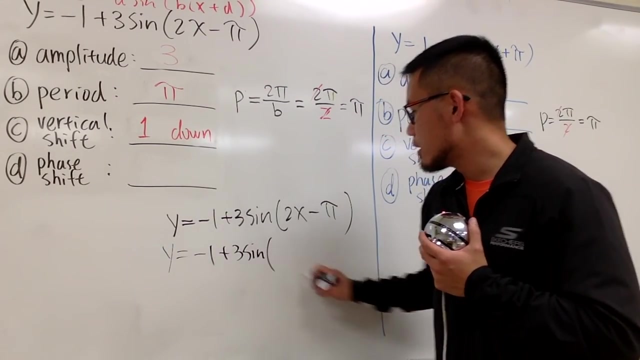 So let me just copy that down again: Y equals to negative 1 plus 3 times sine of 2X minus pi, like this: What we want is okay, everything else okay stays the same: Negative 1 plus 3 times sine. 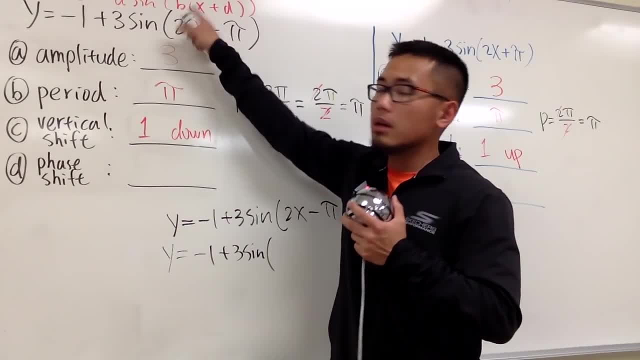 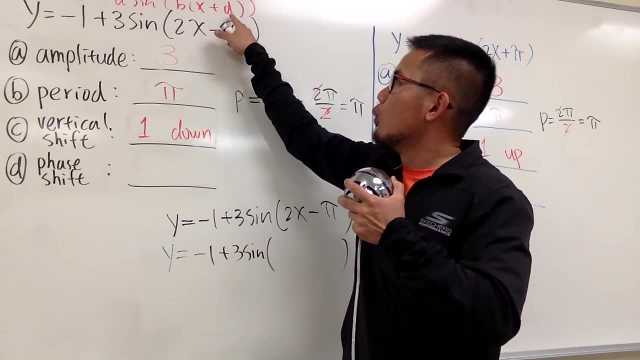 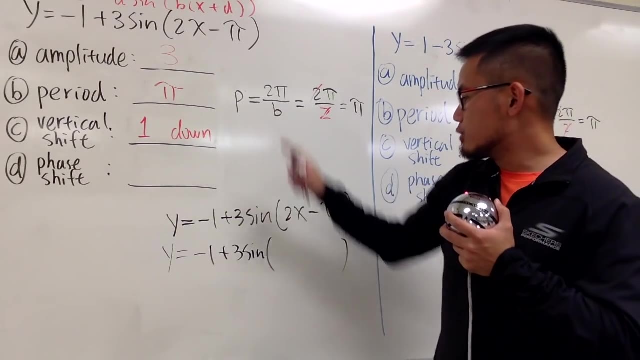 Well, inside we have to make this equal to B being factored out, and then parentheses and X plus D, And the idea is that we need to look at what number is being directly added or directly subtracted to the X. This right here. 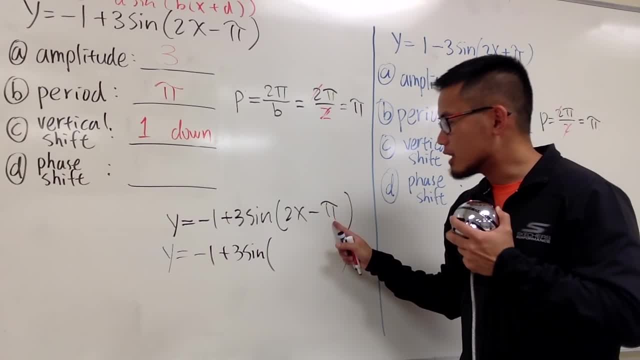 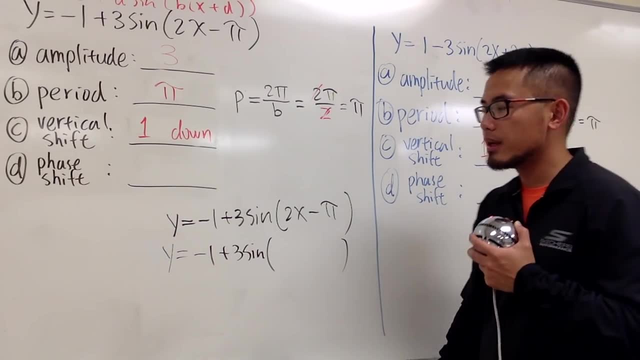 2X minus pi. The pi is not directly being subtracted from the X, because by the Woodruff operation you have to do 2 times X first and then minus pi, right? So anyways, we are going to factor things out. 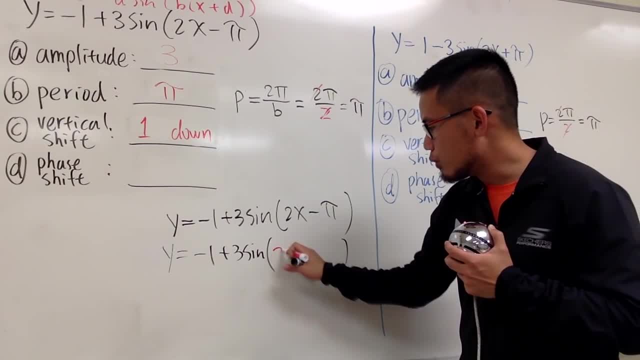 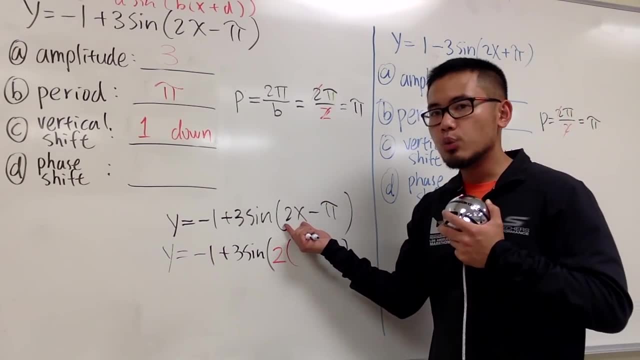 Factor the 2 out. So let me just put down the 2 all the way in the front, first, like this: And then I will open the parentheses like this: And now, this is how you can think about it. Originally we had 2X. 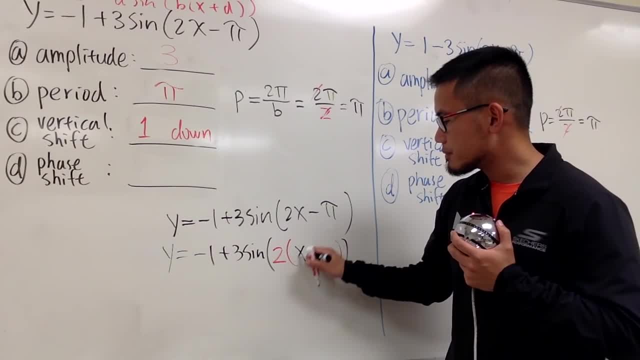 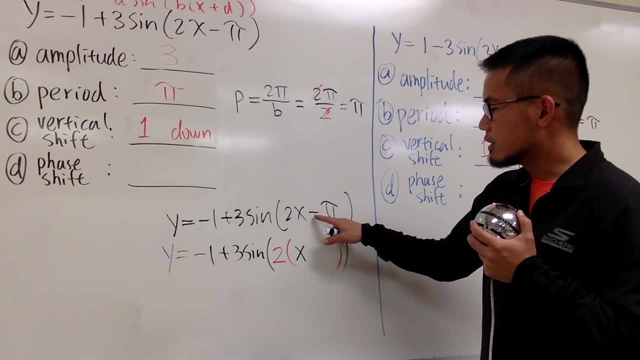 I factored the other 2.. So now we have an X left right here, right, And you can also think about this as 2X divided by 2, you get X. Next minus stays the same because we factored or passed the value here. 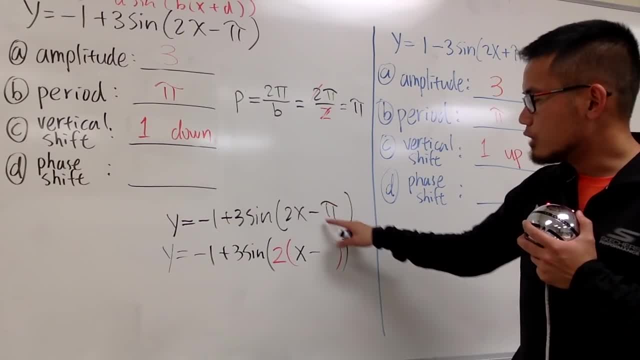 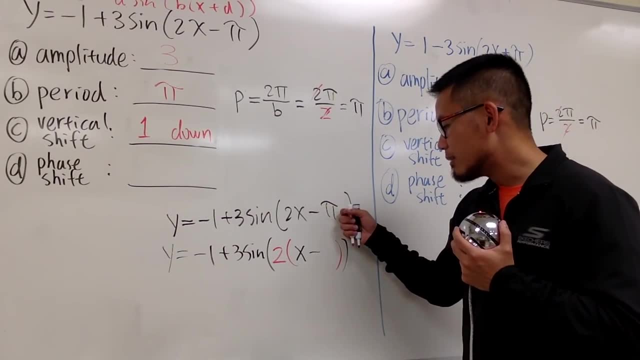 so we still have minus Here. we have originally pi, but then we factored the other 2.. Just think about it divided by 2.. Pi divided by 2, that goes inside, which is just going to be pi over 2, like that. 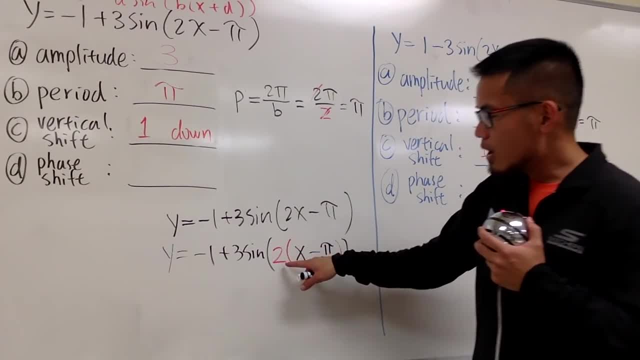 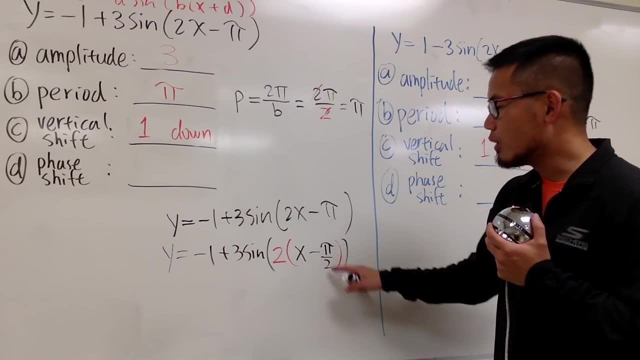 Pi over 2, like that. Well, you can also always do a quick check: 2 times X is 2X, 2 times negative pi over 2.. The 2 will cancel and you end up with negative pi. 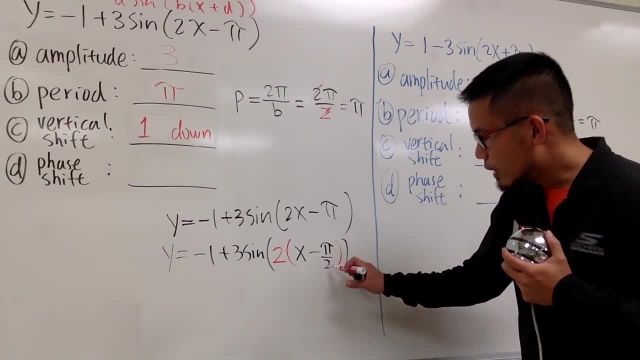 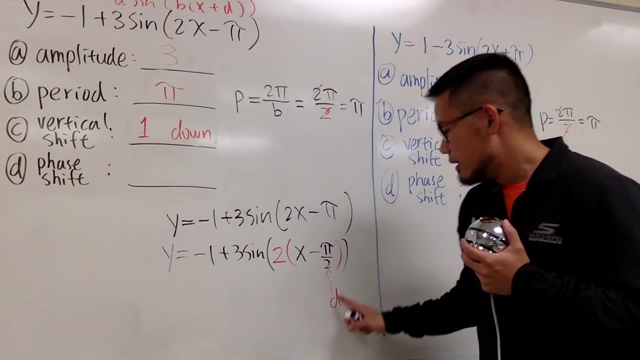 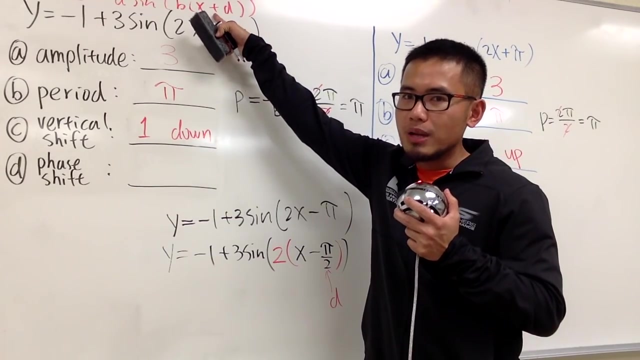 That means your factor is right. This right here will tell you the d value and it will tell you the phase shift. all right, But let me just not write this down: the d value, because this right here you see, original formula is plus d. 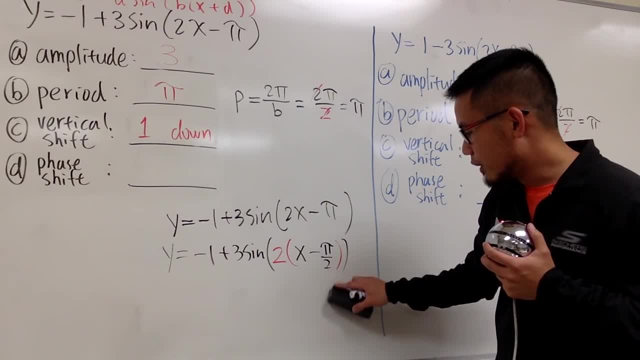 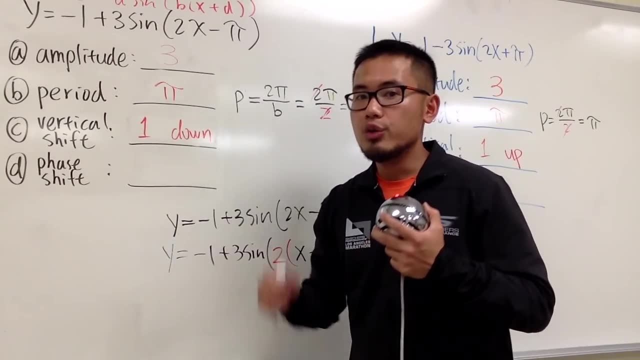 This right here is minus pi over 2.. But this is the d value. I just want to point it out right here. Okay, for the phase shift, it's similar to the vertical shift. You're going to tell me however many distances we're going to move. all right. 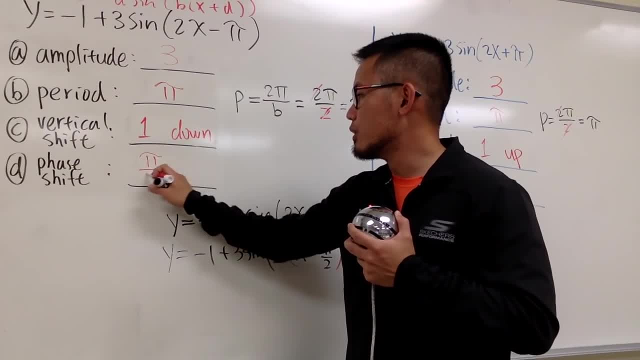 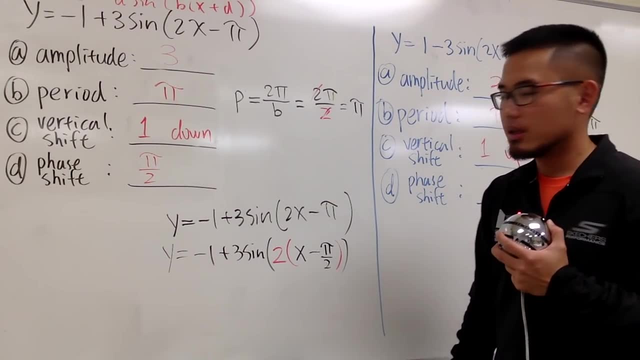 It is going to be pi over 2, regardless to the direction. at the moment, The value Y is just going to be pi over 2.. Next, you identify the direction. The phase shift is going to be left or right because you are adding or subtracting. 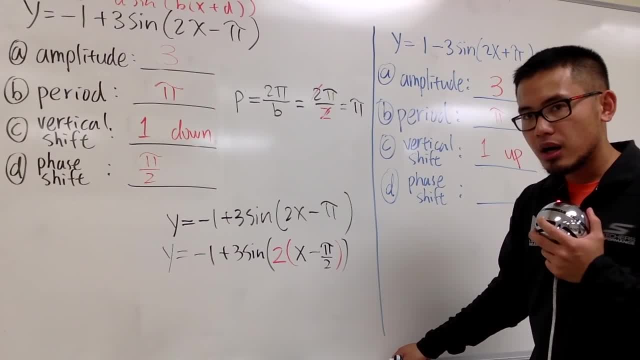 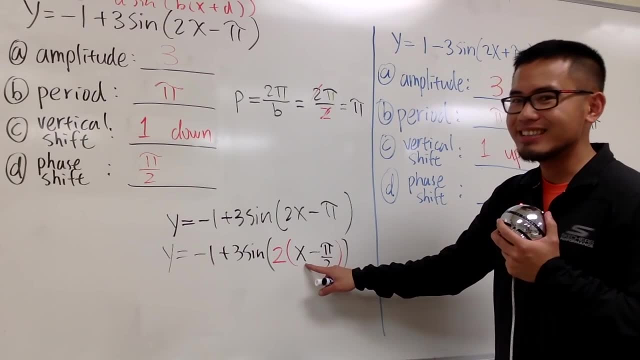 directly toward the X. Here is the tricky part: When you are directly subtracting pi over 2 to the X, subtracting pi over 2 to the X, you're actually going to move toward the right. So it's the opposite of what you see, right. 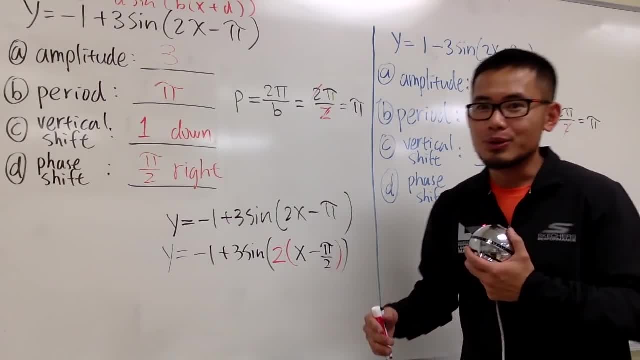 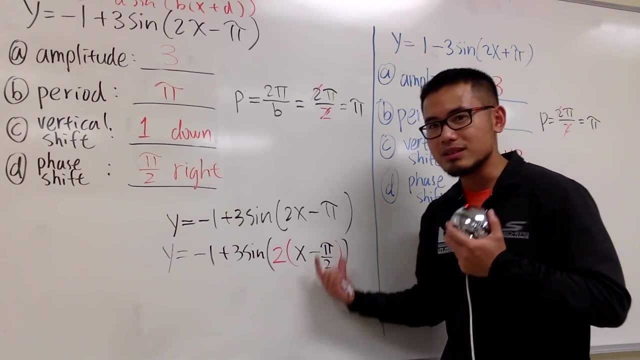 Because normally you associate negative being, you know, to the left, and then positive toward the right. But now, when you have this in the parentheses, when you have this in the parentheses, it's the opposite. When you see negative pi over 2,. 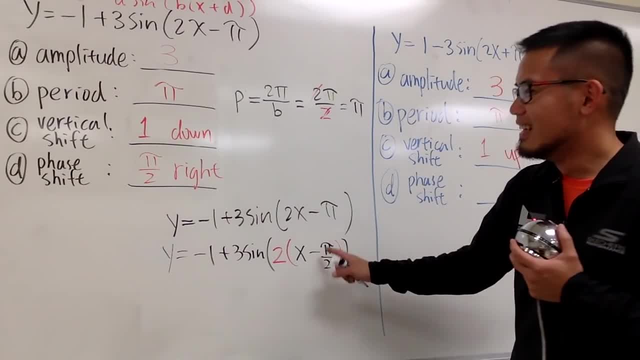 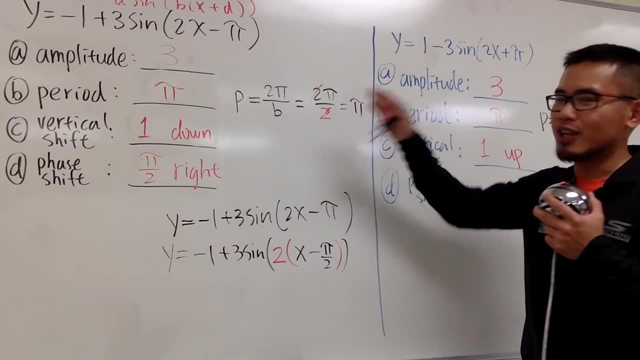 it's actually moving to the right. all right, Okay. On the other hand, when you have 2X plus pi, you know the comparison already. I just changed the signs right, But anyways, let me put that down right here. 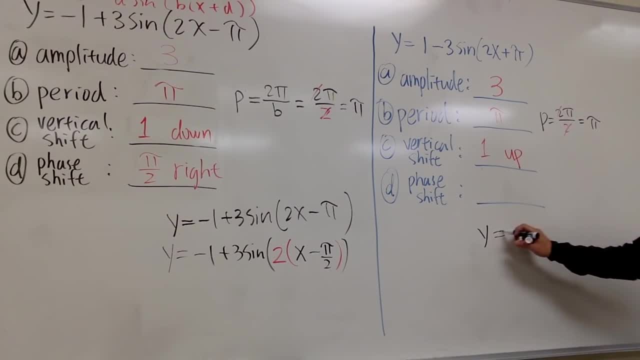 That will be: Y equals to 1 minus 3 times sine, And let me factor out this 2 right here for you guys already. So I put down 2.. And then it will be very similar to that which is X plus. 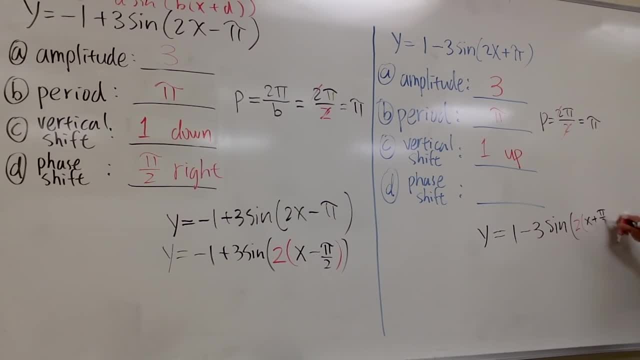 X plus pi over 2, like this. Okay, I'm not going to tell you what the default value is, because that's tricky. You just have to tell me however many units that you are going to move. right, So it will be once again pi over 2.. 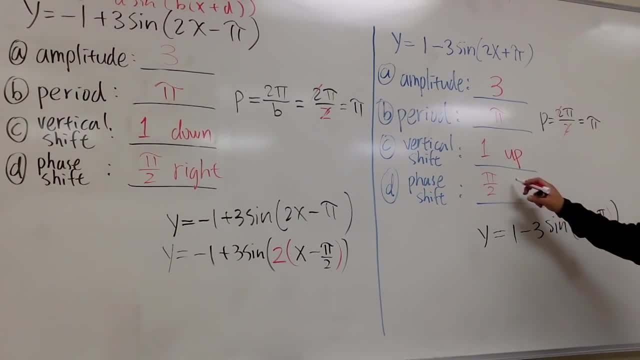 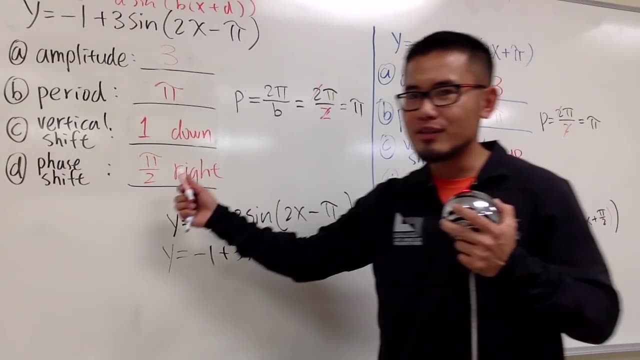 But this time, when you are adding directly to the X, it is moving to the left. So pi over 2 toward the left. Earlier it was pi over 2 toward the right. So be sure you study and remember all these details. and that will be wonderful. That's it. 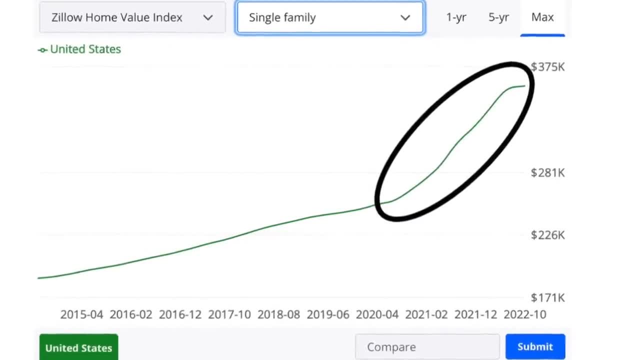 Many are calling this the largest bubble in US history. Following three years of greed, speculation and easy money, the US housing market is finally starting to show concerning fractures. While many on YouTube are quick to point out that prices remain high, fresh new data shows that we're entering a housing crash that could cause irreparable damage to the markets.